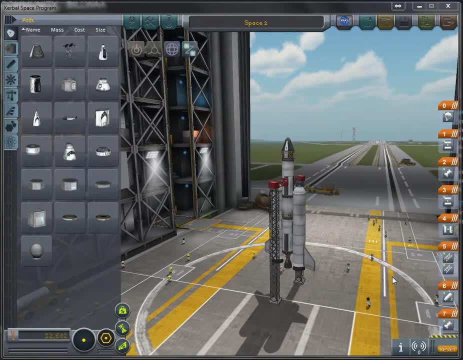 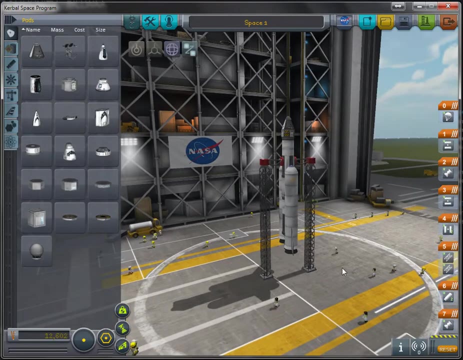 Hi, this is Billy Ho. We're going to go over some of the mechanics here. Instead of using notes and PowerPoint, let's use the Kerberos space program, because it's much more fun this way. So here we have our rocket. We call it Space One, And our rocket here consists: 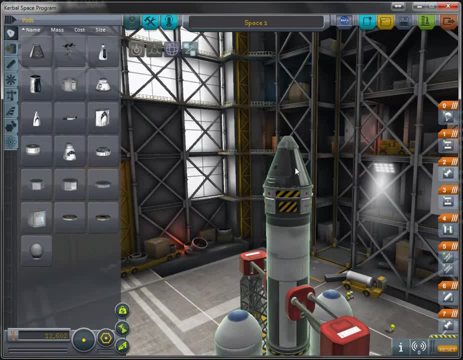 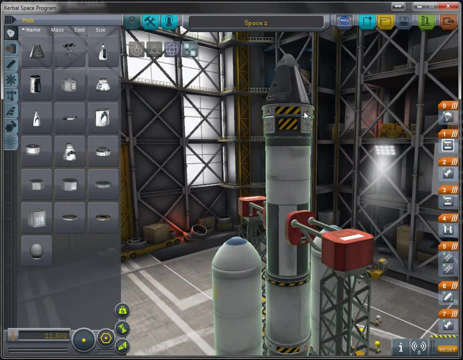 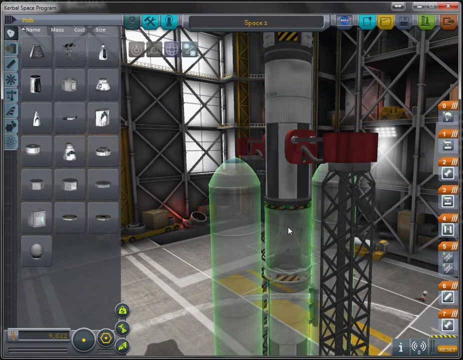 of crew capsule and we have a parachute for the reentry and landing. We have a separator here to separate the crew capsule from the rest of the rocket. We have a reaction control wheel thing here- This is the second stage- fuel tank And then we have a rocket engine. 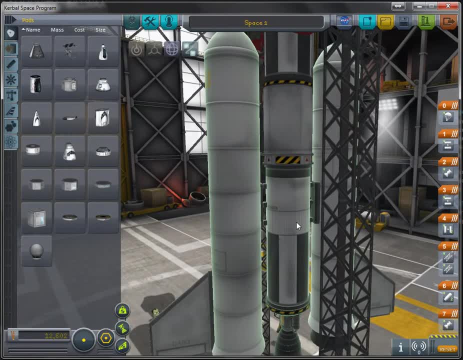 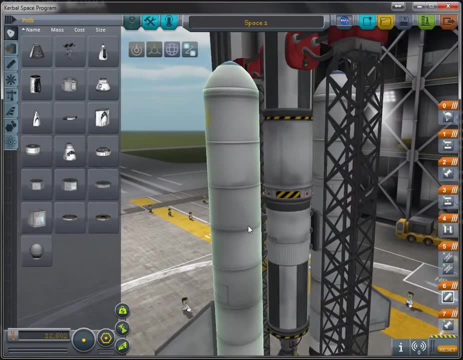 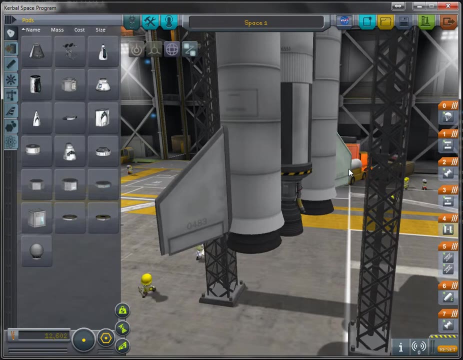 in there. attached to that We have another separator, first stage fuel tank And then rocket engine. We have two solid rocket booster attached to the rocket. Those are separator to separate them. Then we have two wings to add. you know our attitude: control, Okay. 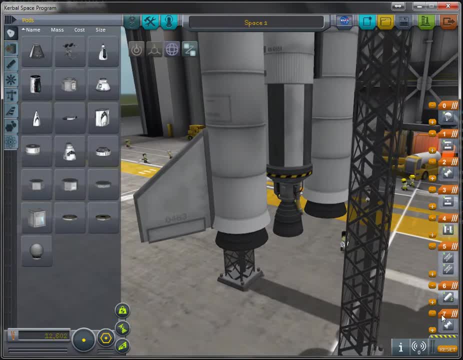 So here we have our staging setup. First we're going to turn on our cryogenic rocket on this first stage. Then we're going to turn on our solid rocket booster. Now, the reason why we're going to do it this way is because the solid rocket booster is going to be a 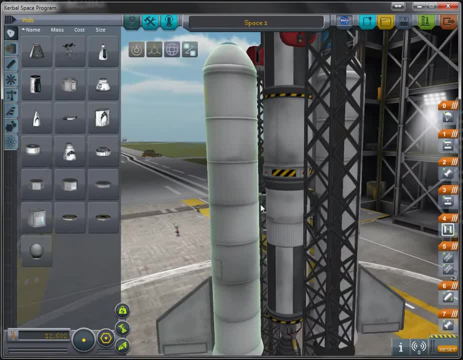 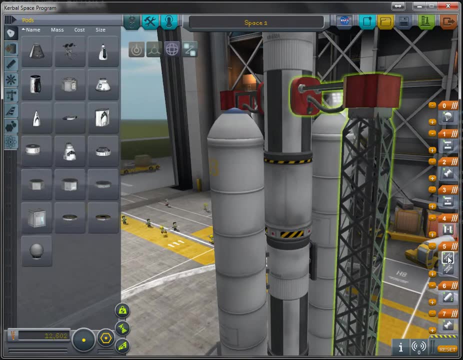 little bit harder to turn on. So the solid rocket booster: once you start them, you can't turn them off. That's why we want to turn on the cryogenic first, to make sure that everything's working right. So after that we're going to release our clamps. So you know we have. 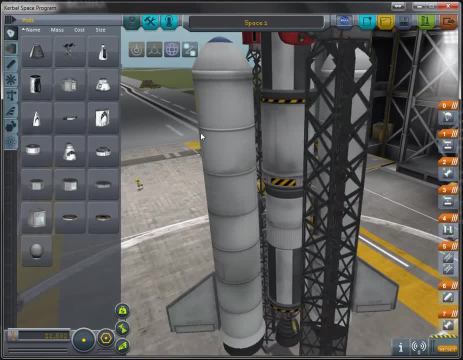 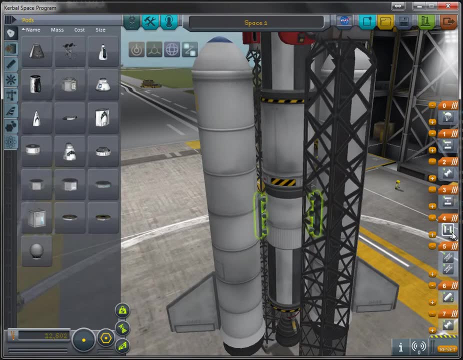 to lift it off, And at a certain point the solid rocket booster is going to burn up. So we are going to separate them by activating the separators, And then at that time, our first stage is just about to burn up too, So we're going to separate that with the. 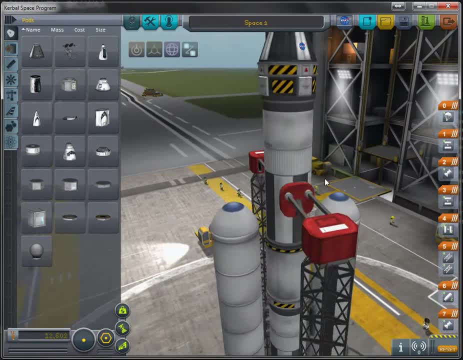 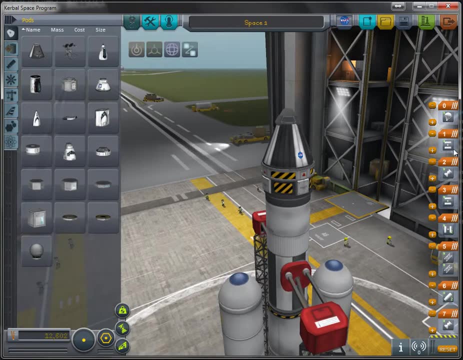 with the rest of the rocket we're going to ignite and launch, start the second stage cryogenic engine. so after that's burned out, we have another separator to just you know, separate crew capsule with the rest of it and we're prepared for the entry landing. so let's launch. 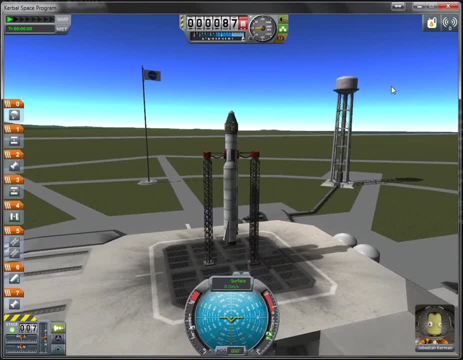 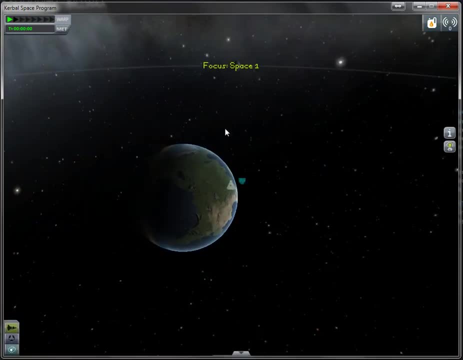 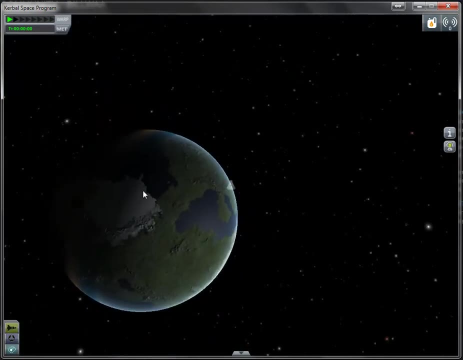 all right. so we're at the Kerbal Space Center right here. let's see, we're almost ready for launch. let's look at the map real quick. so this is our solar system. we have, well, our planet, Kerbal, Kerbin, whatever- i don't know how you call that- basically earth. then we have a moon. we actually 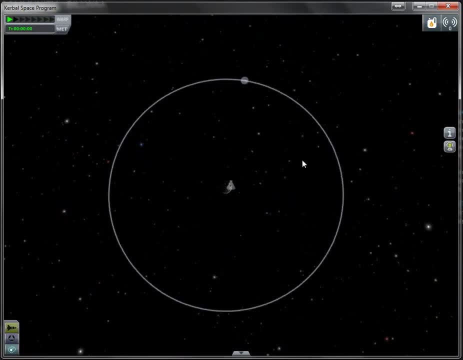 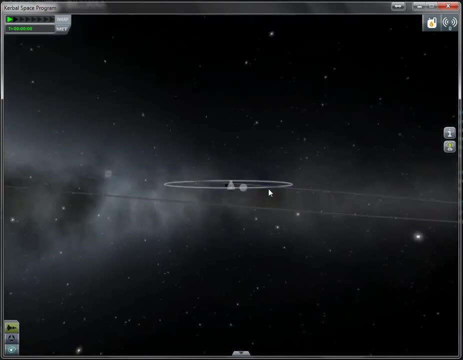 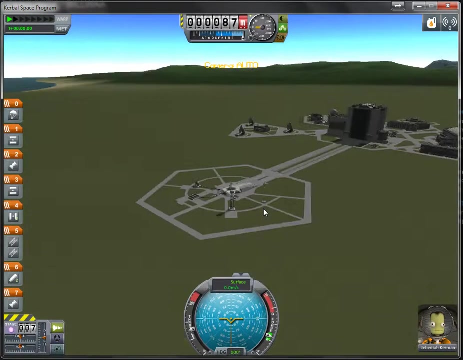 have two moon in this system. the first moon, as you can see, is in the basically the same plane planet the same planet. i can't move this. uh, no incline, we have incidental inclination. anyway, let's go back here. so the plan is: we're going to lift off and we're going to 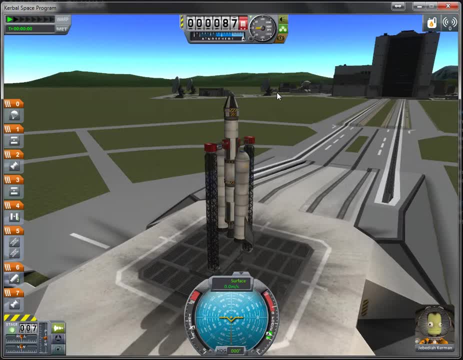 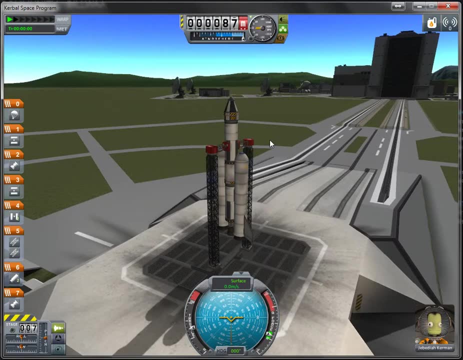 go vertical to gain some height. so until we reach 10 000 meter we're going to do a row to around 45 degrees. that will put us into a more parabolic trajectory, where then we can do our orbital maneuver to achieve orbit. all that so okay, let's turn on our reaction control system and stability. 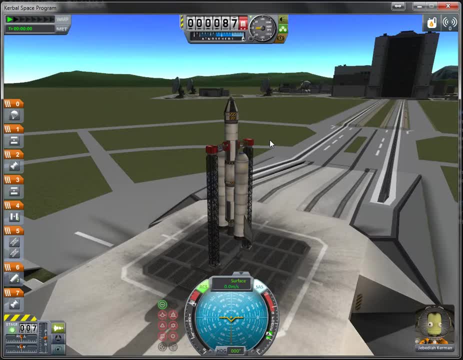 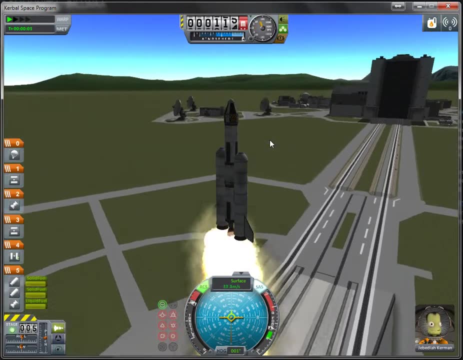 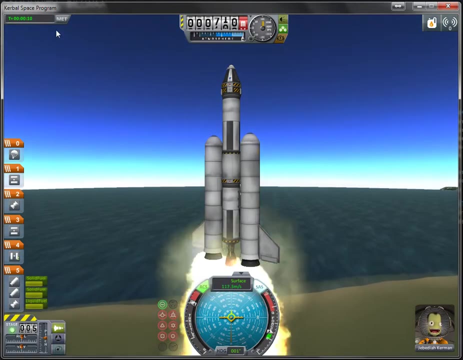 application system, follow-up and start the cryogenic engine. that's good. rocket sound like a booster is on and lift off, all right. so this is gonna take a while. this is just gonna go up. I tried doing the warp drive earlier and the whole rocket fall apart, so she let that run a little bit. 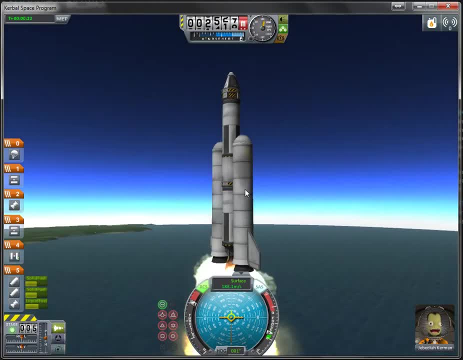 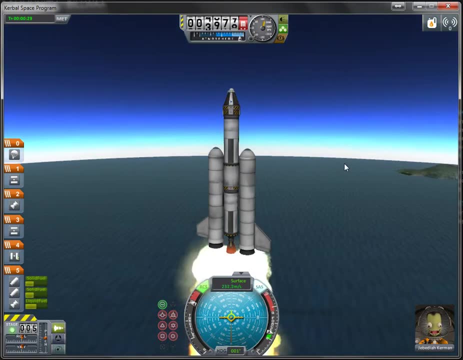 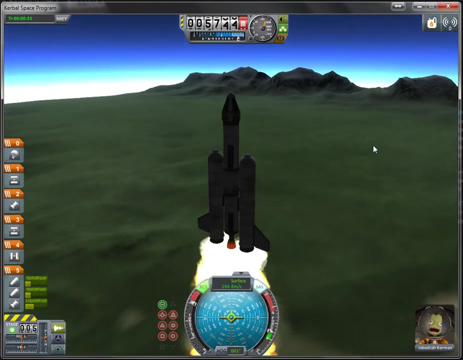 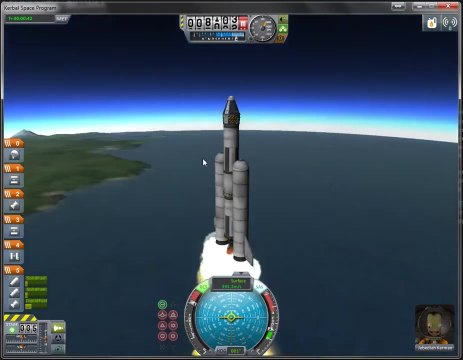 okay, you see the moon here, we'll try to get there. well, not get there, I'll show you how to how you can plan your burns to get there with this rocket and dark enough propound to get there. you all right? so our soil, I can push that ball. the burnt-out we gonna separate. 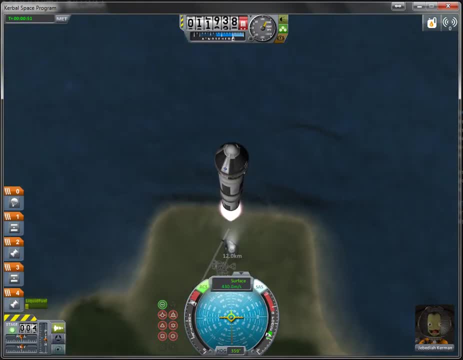 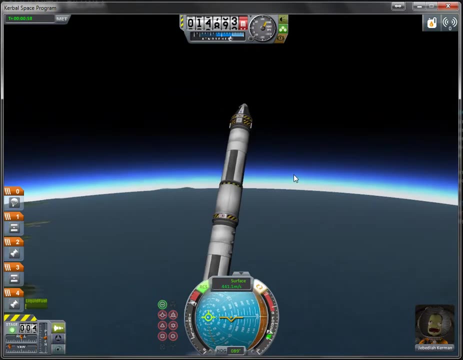 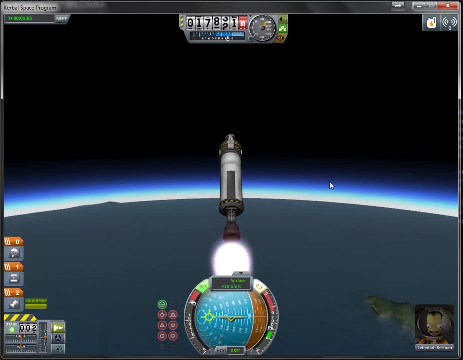 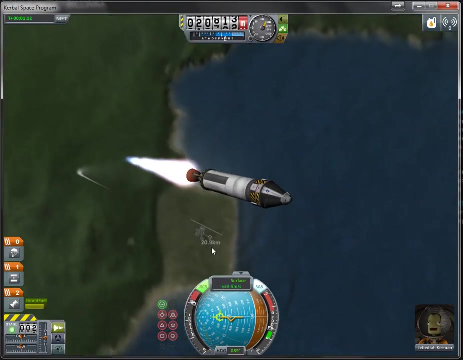 them all. right, did that? yes, and I talked: okay, that's right on the center. okay, let's do a roll here so you get away from land. other sweet much okay. second stage: okay, so that shouldn't cost much0. gonna crash right back there. that's someone else's problem. okay, let's look. 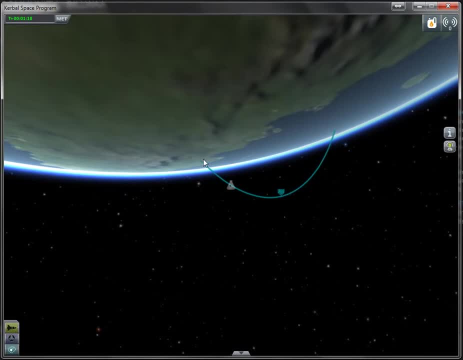 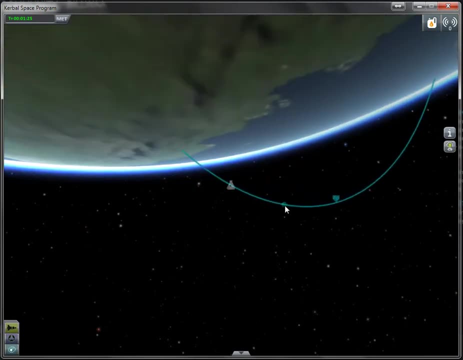 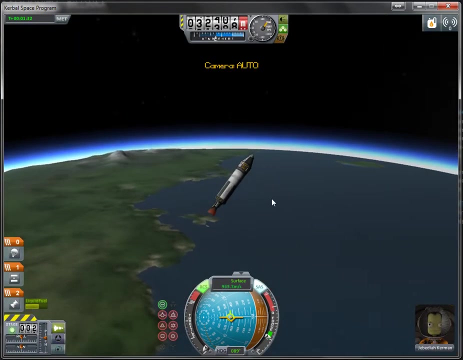 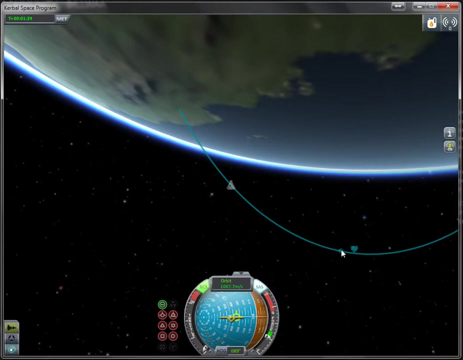 at our trajectory. you see, right now we go from like a, you know, straight up, straight down to a more parabolic trajectory and, okay, to save some fuel, we go to stop right here. how much fuel we have left? all right, a little bit more, half, okay. so if you remember from me, 255, intro, aerospace engineering, you know, 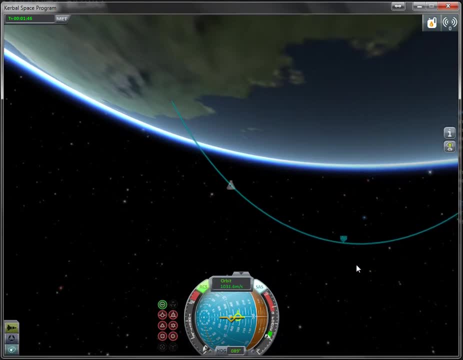 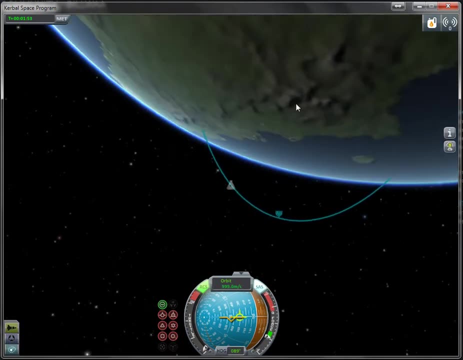 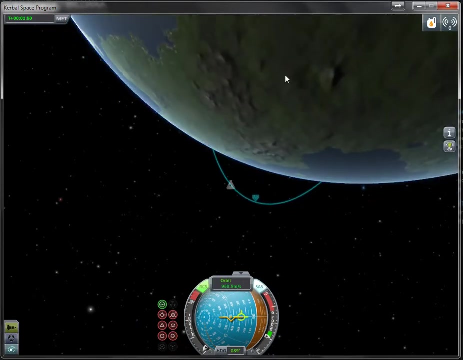 well, the highest point of a orbit is called a palace, which were here. since we are not really in orbit right now, our pair Alice is like right there on the ground. we want to raise the palace pair Alice to a higher altitude so that we could achieve orbit. so how we do that is we. 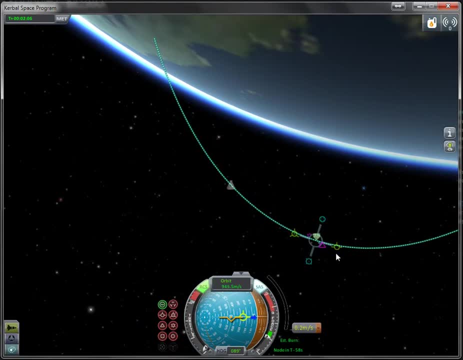 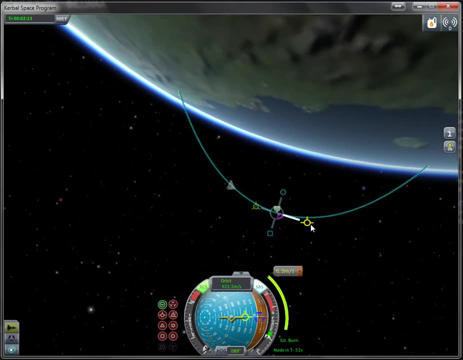 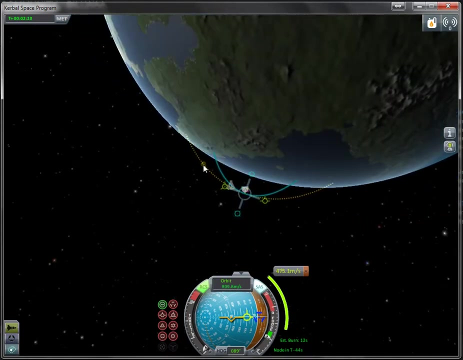 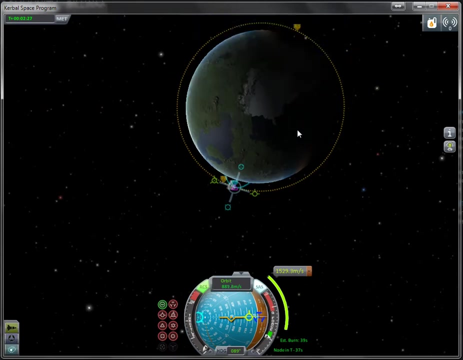 do a maneuver at a palace and then we thrust program, which mean you want to thrust along the velocity vector so you can see we first you know 400 meter per second track. you get wider. so basically you want to do this until you are in a circular orbit. you can think of it this way. basically you keep your basic. 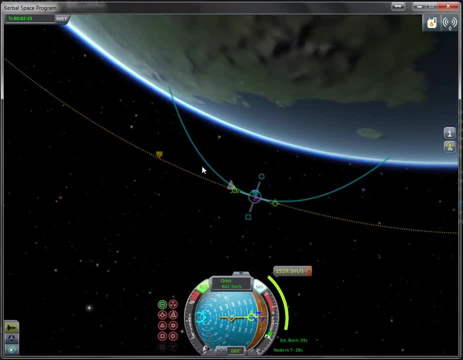 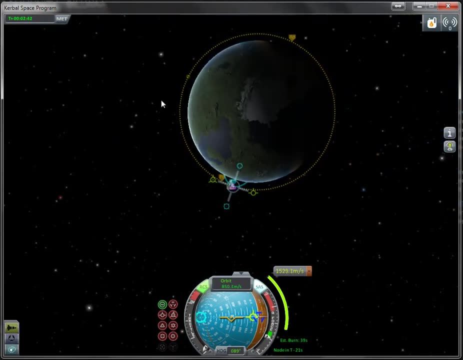 falling right. so the faster you go, you can go four farther, and if you go fast enough, you you keep falling, but you misses the earth, and that's how you achieve orbits right here. anyway, since this is not SDK, take time to do a burn. we need to burn. 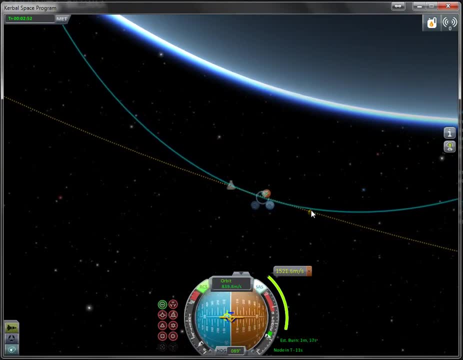 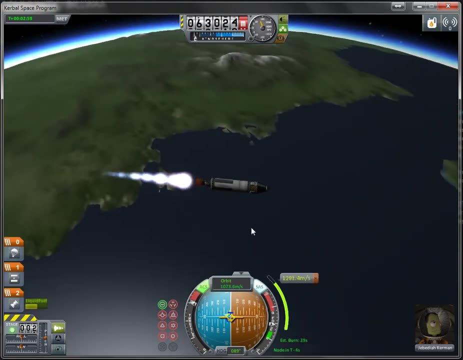 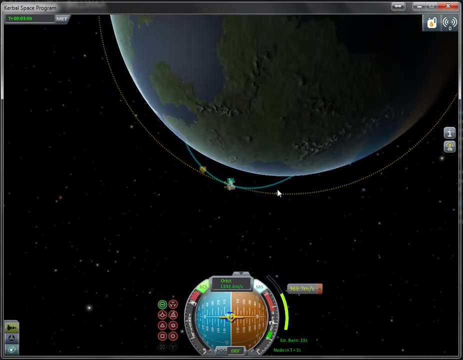 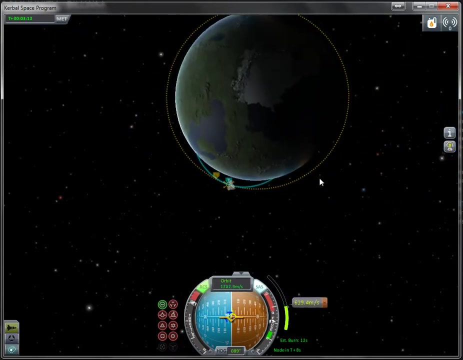 now and let's see aim to our target and burn and wait. is that? yes, okay, so you can see we pretty much burn the impeller with the ground and a street burning. you can see that our orbits is scaling, less elliptical and more circular, so it's burning, Burling, burning. 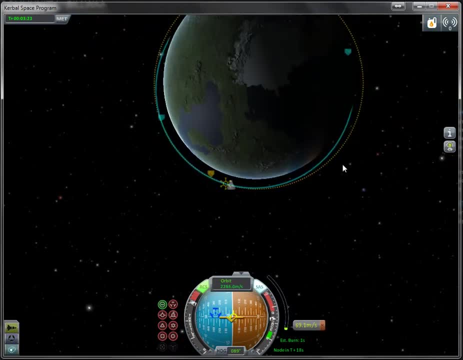 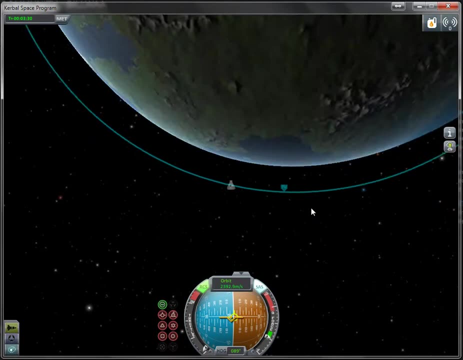 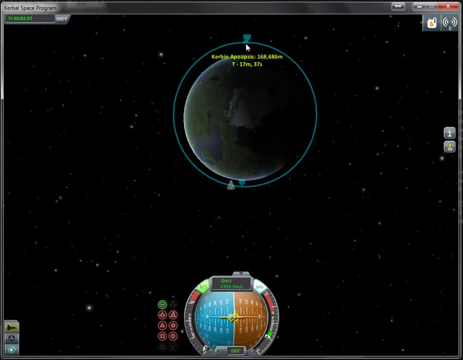 all right, that's about enough. all right, all right. so you said: burn a little bit, All right, that's about enough. the parallel is actually switch location because now, since we burned that much out, this point of the orbits is actually higher. so that's why that's the new apparatus and the new paralysis right here. 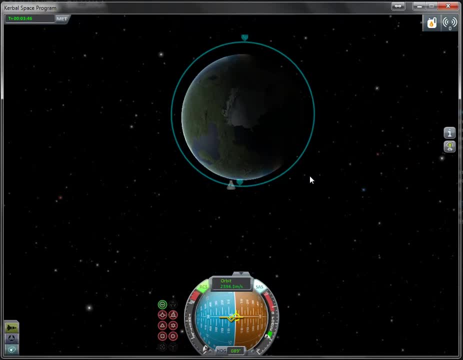 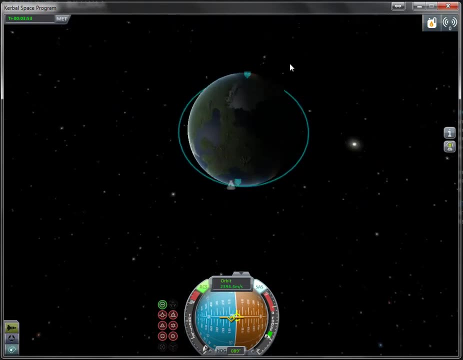 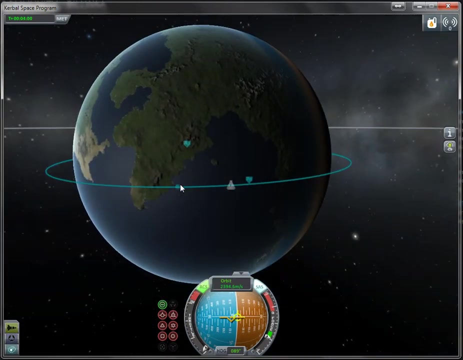 okay, so now we know how to do our maneuver. uh, you know, changing orbit. let's um, do a little bit more advanced stuff. um, okay, so let's say that we want to change our inclination. see, right now we're in like a equatorial orbits like which, which is like along with the equator. 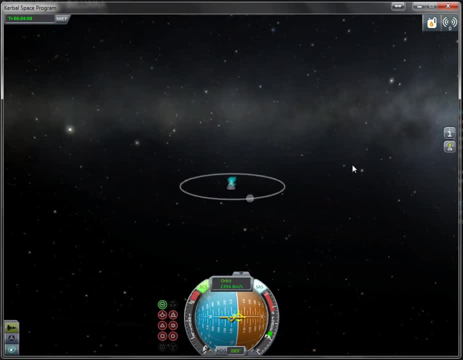 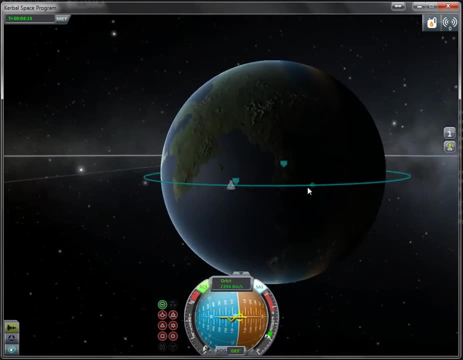 uh, let's say we want to, you know, go to the second moon, which is, you know, totally in a, not in like a different inclination. um, what we would do is we would pick the ascending node or descending node, and i don't know where that is here, so i'm just going to pick a random point. 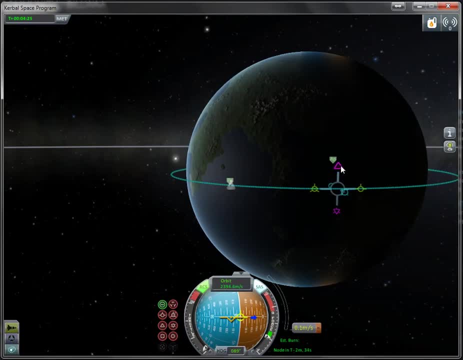 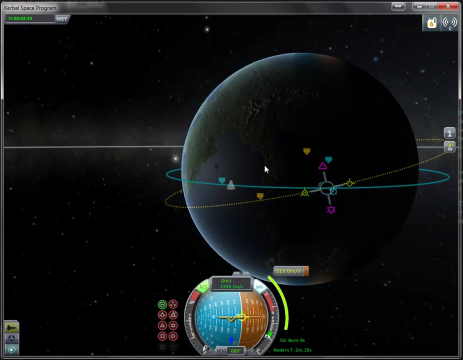 add a maneuver. so if you thrust upward or downward with respect to the inertial frame of the planet, you can actually change the inclination like that. so, uh, changing inclination should use a lot of um, delta v. so a better way to do that would be when you launch. you launch into a certain 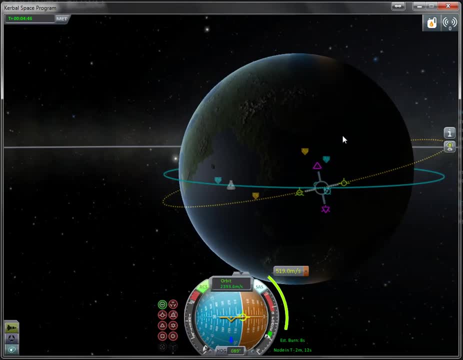 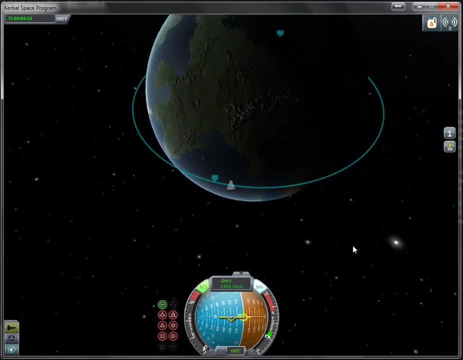 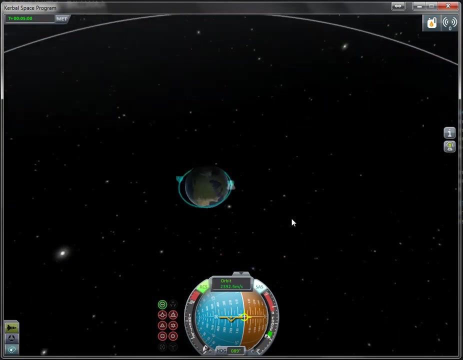 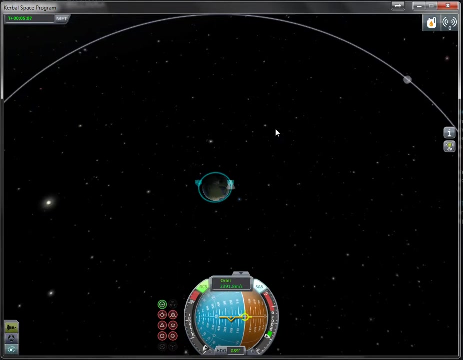 inclinate, like inclined orbit. so you don't do this inclination later on. it saves you some fuel. so that's how you do inclination change. um, let's try to get to the moon. one yeah, moon, okay. so what, um, we're going to do is a simple holman transfer. basically, how that works is that we 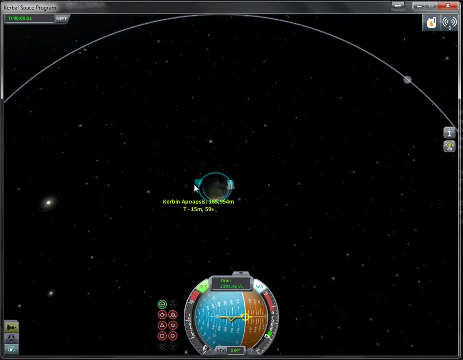 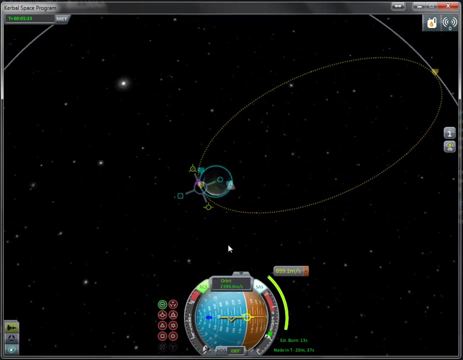 pick a certain point in our orbit and we do a delta v maneuver. though okay, let me just do it, let's pick this point right here at maneuver and we'll flush prograde that will put us into a highly elliptical orbit. basically, this is our transfer orbit to transfer into a high orbit from. 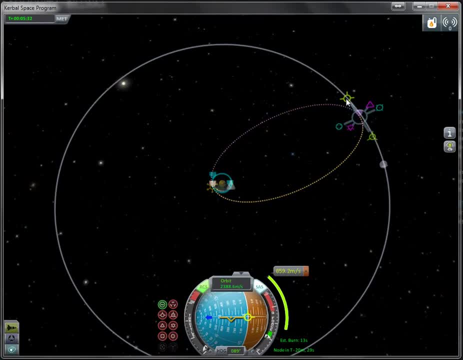 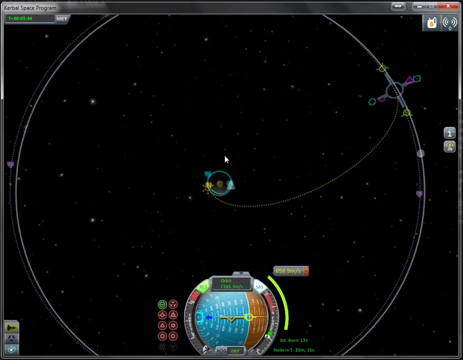 the moon. here we could basically add an iron and we refer and we can basically, you know, flush, prograde and that will bring us to a bigger orbits right here. see, this is how we do a holman transfer from a lower, low, um, well, low, earth orbits, low carbon turbo orbits, to a high 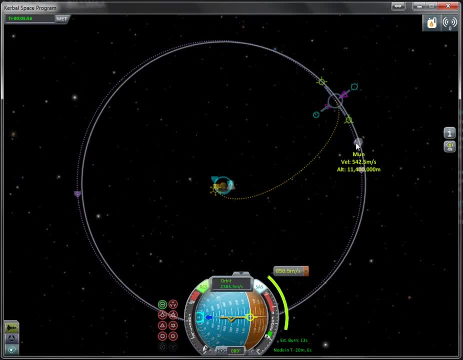 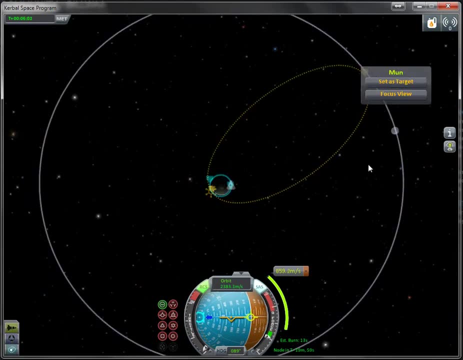 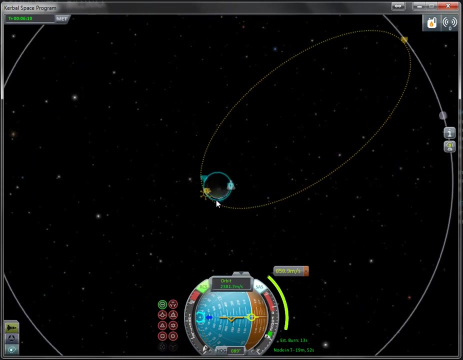 orbit right, like this, okay, um. but since we want to run the rule with the second burn, well, we need a second burn, but not like this, okay, um. so, as you see here, right now, when we get there, the moon is not there. so we need to basically pick a point. 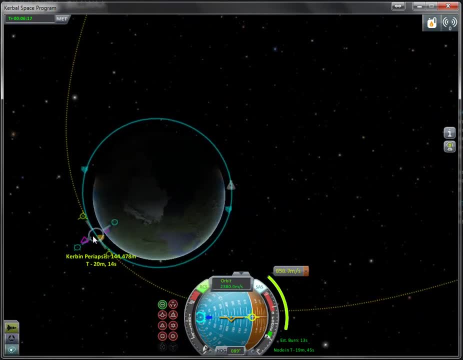 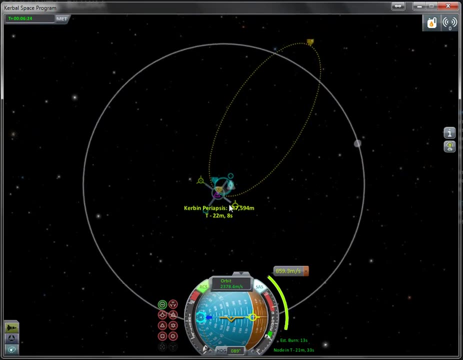 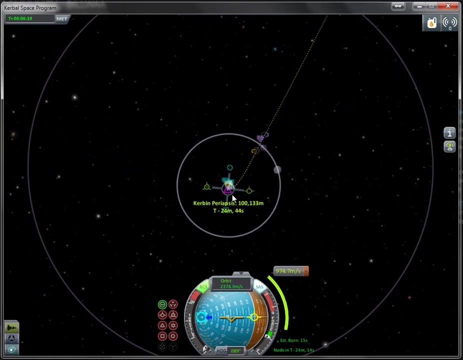 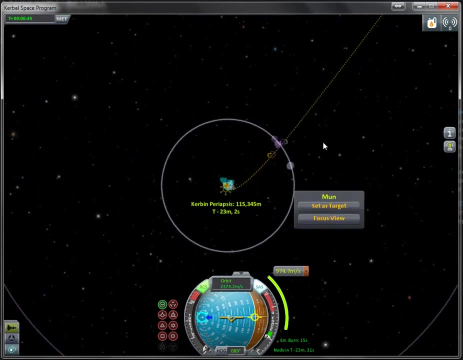 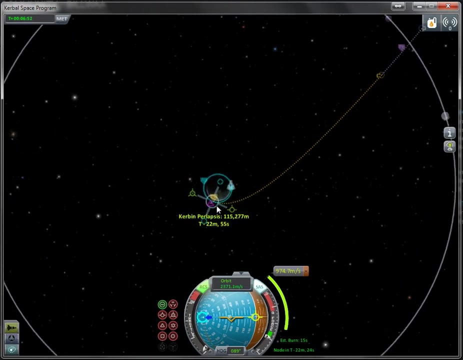 so that when we thrust, uh, the moon will be there. so let's move this maneuver. let's see, all right, uh, right here. all right, so you can see that when, if we thrust up, no, um, um, okay, i screwed that up, but um see if we can get that back. 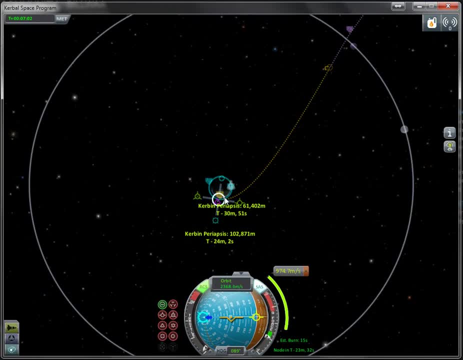 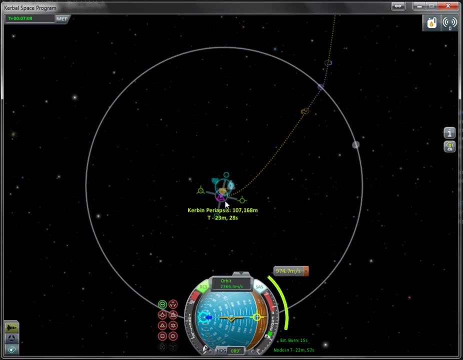 okay, that's good, all right, so let's okay, this somehow, okay, well, anyway. so then, uh, when we do this maneuver, when we get to this point, the moon will be there and since the moon have some sort of um gravity pull right, it will basically um pull us with it to see our 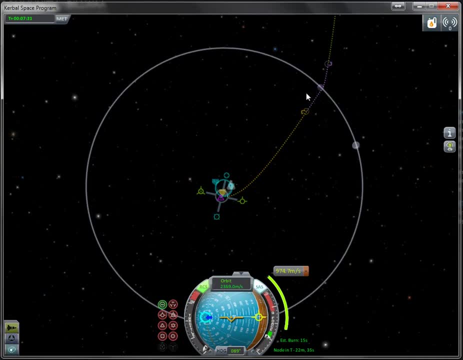 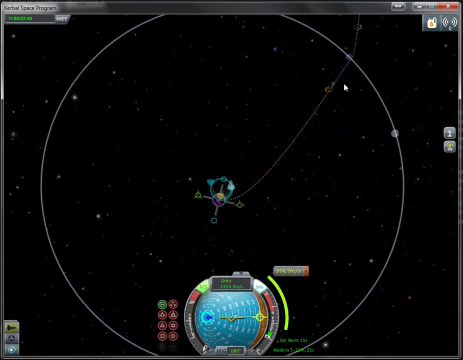 original trajectory this way like: oh, actually it's fallen like this, right. however, the moon is here, is pulling us there, and then alter our trajectory and shut us like way outside farther into the solar system. so this is like a gravity assist maneuver: if we want to orbit around the moon, um well, this is way too fast for us to actually orbit around the moon. 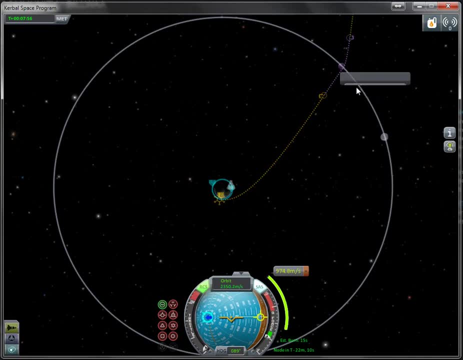 what we need to do is we need to add a maneuver. so we add a maneuver here and we thrust, thrust, retrograde. you know, anti-velocity vector. when we do that it slows down and you know, the slower we go when we get to the moon, um, the more the gravity, uh, the long like, basically, they.